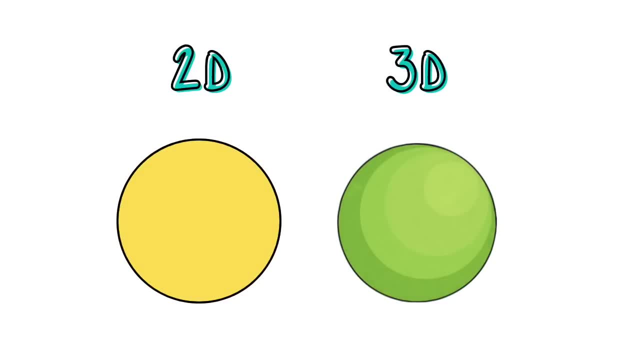 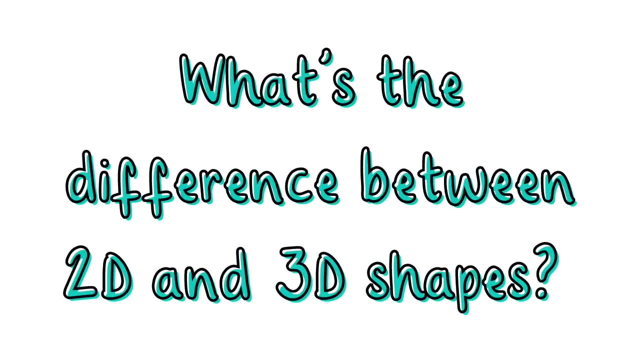 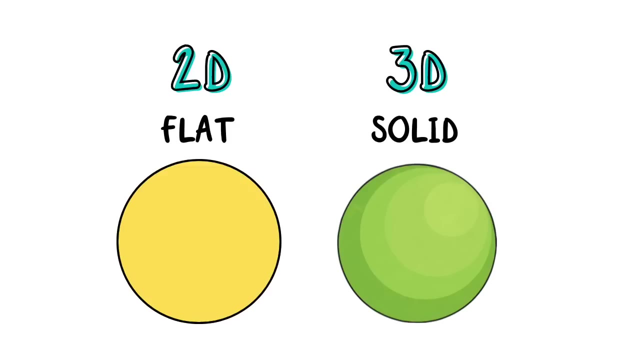 But today we're going to focus on recognizing 2D and 3D shapes and study their properties. What's the difference between 2D and 3D shapes? One of the easiest ways to understand the difference between 2D and 3D shapes: 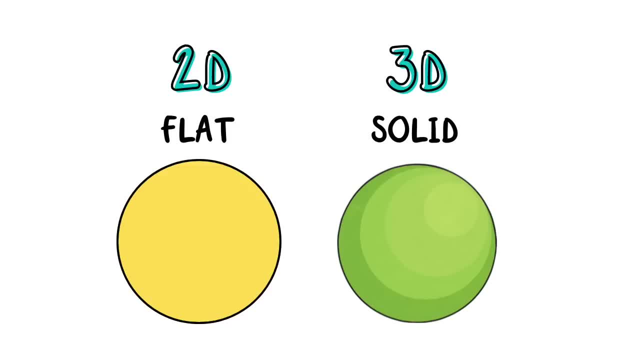 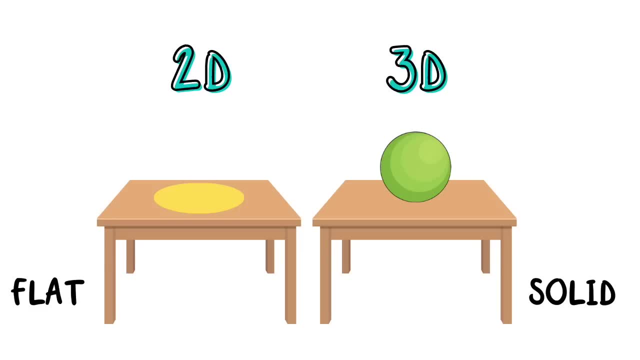 is by identifying how 2D shapes are flat and 3D shapes are solid. For example, if you place a 2D shape on a table, it will lie flat on the surface. If you place a 3D shape on a table, it might roll or stand upright. 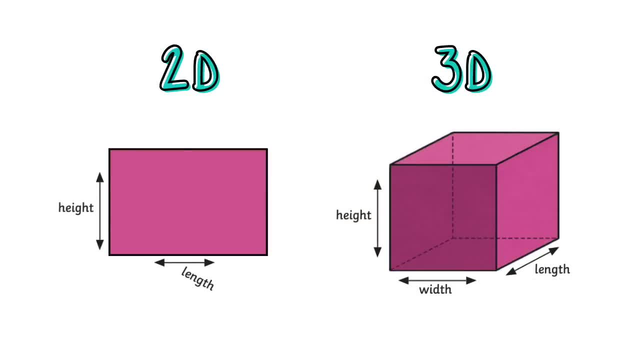 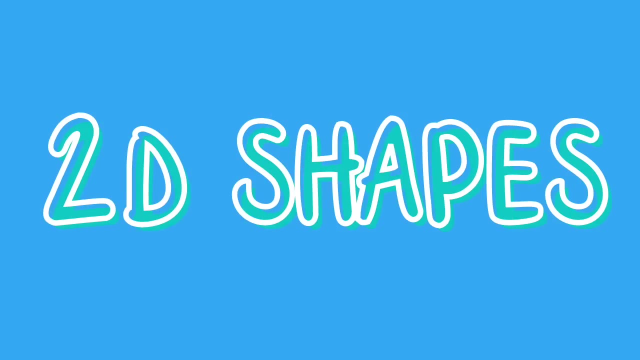 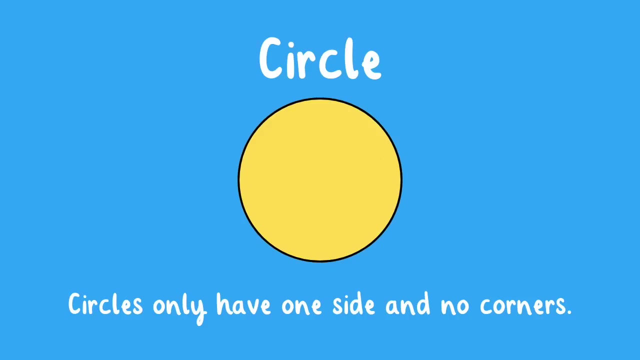 Furthermore, a 2D shape has only two measurements: length and height. A 3D shape has three measurements: length, height and depth or width. Now let's take a look at some 2D shapes. Circle Circles only have one side and no corners. 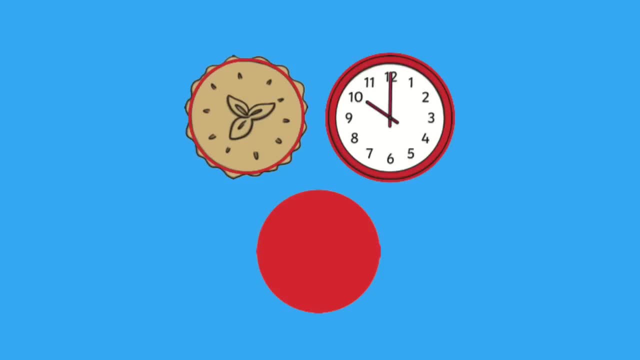 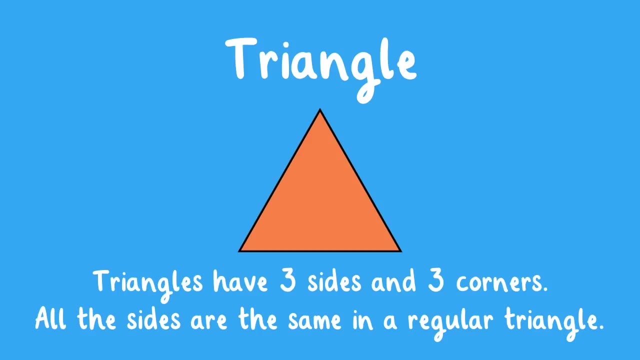 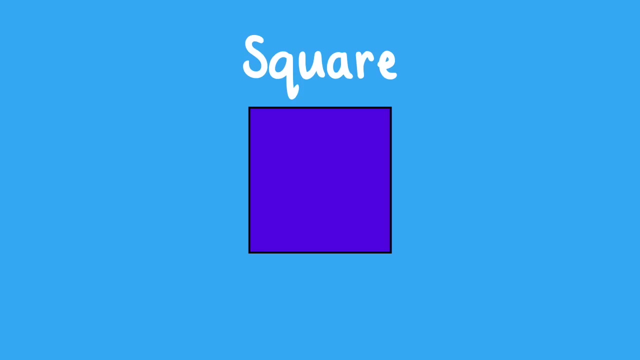 Here are some real-life examples: Triangle Triangles have three sides and three corners. All the sides are the same in a regular triangle Square. A square is a regular shape. It has four straight sides and four corners. All the sides are the same length. 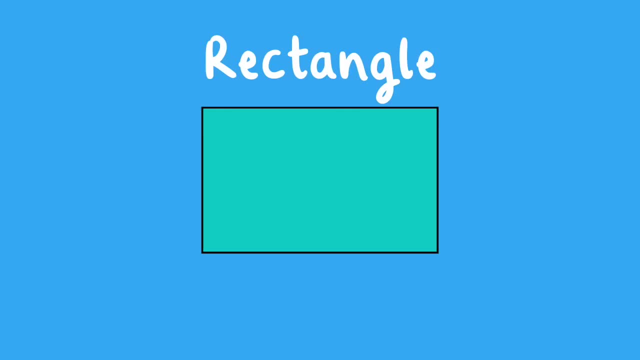 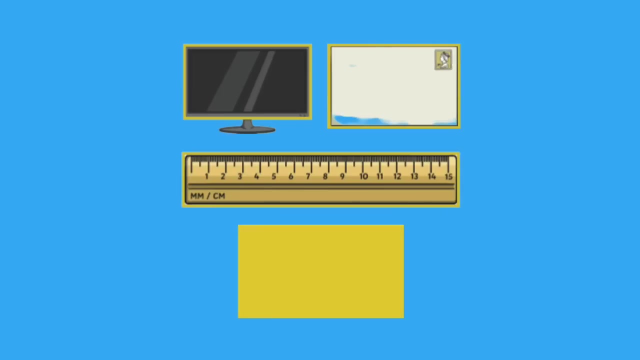 Rectangle. Rectangles have four sides and four corners. They have two long sides and two short sides. This means that a 2D shape has two straight sides, a semicircular shape and a rectangular shape To equate the axes. actually matching cutbook shapes can be done. 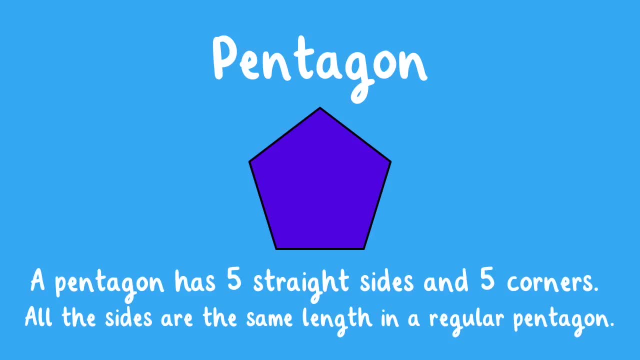 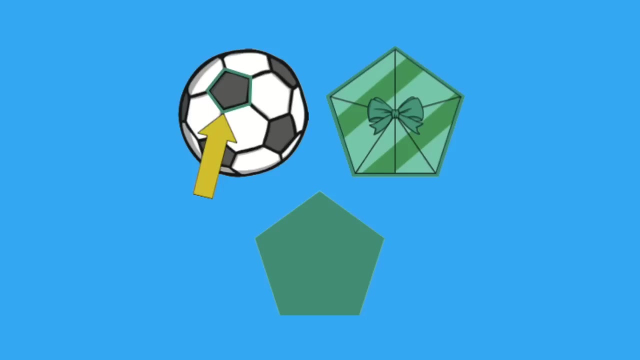 Colour. A colourful squirrel must match three different colors, So I used a oggi projections pessiogue. Pessiogue has soft and contenidoed 근ci: launches Vertical surface. Vertical surface sweep. so are找eptics. 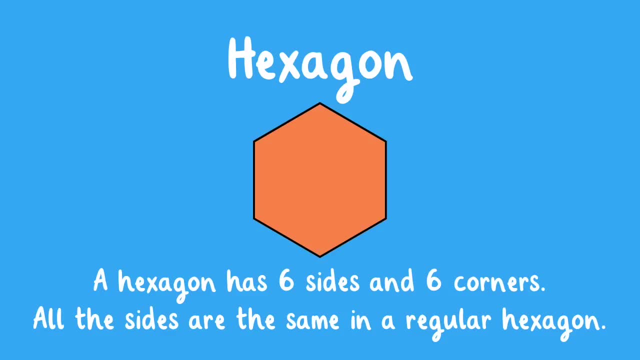 meterogastaires can. pentagon, pentagon- pentagon, Pentagon- has five straight sides and five corners. Perihlert indexes have five straight sides and five corners. All sides are the same length in a regular pentagon. six sides and six corners. All the sides are the same in a regular hexagon. 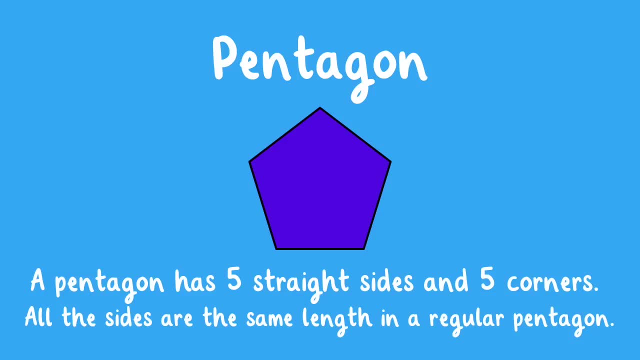 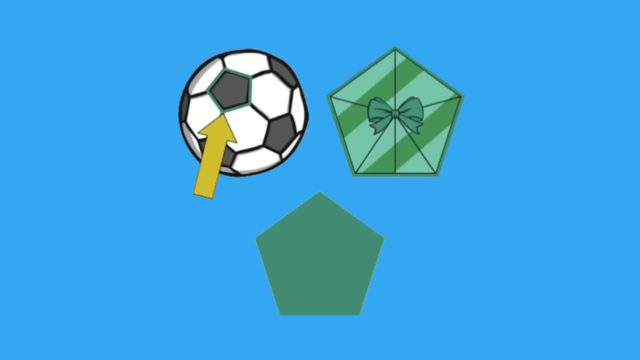 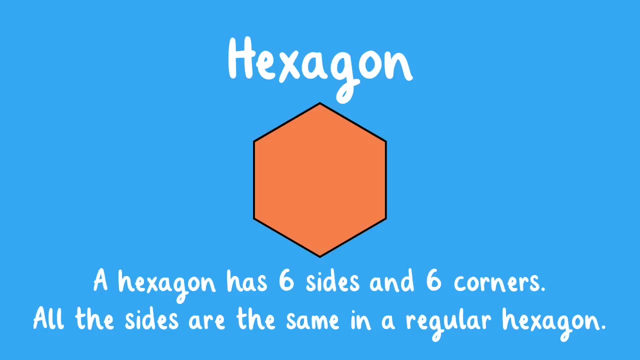 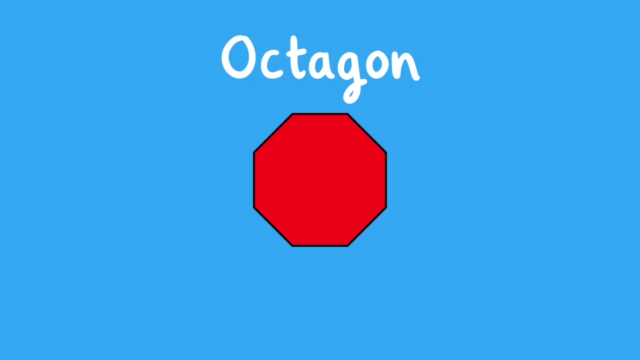 Symbol: Pyramid. A large slide has three sides and two corners. All the sides are the same. in a regular pentagon Pentagon. A hexagon has six sides and six corners. All the sides are the same. in a regular hexagon Octagon: An octagon has eight sides and eight corners, All the sides. 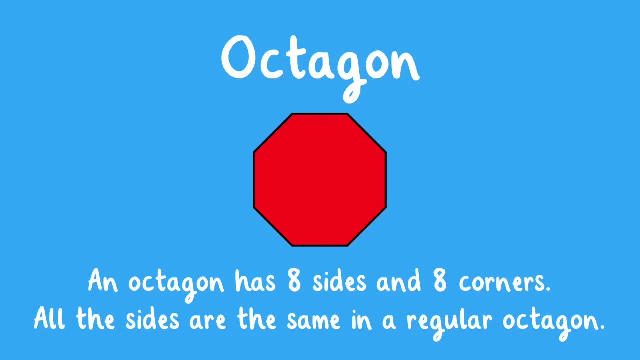 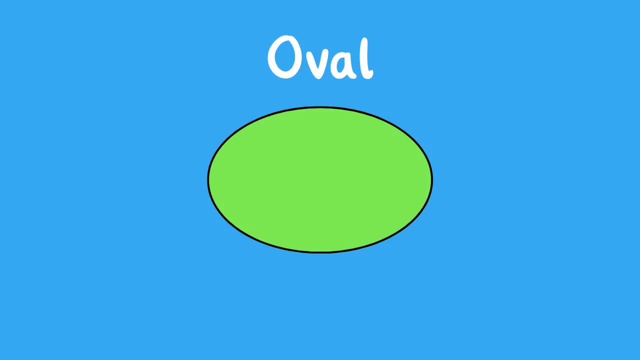 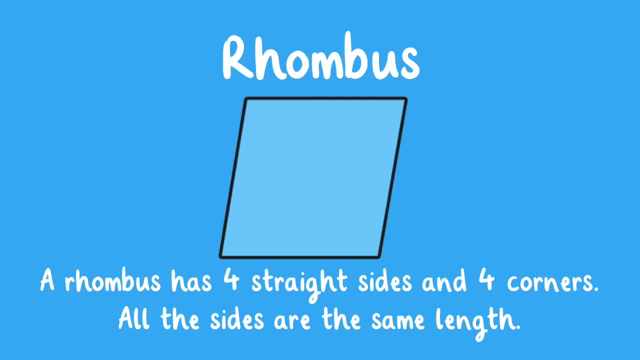 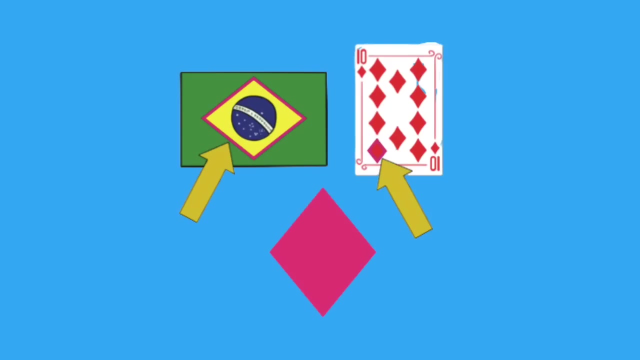 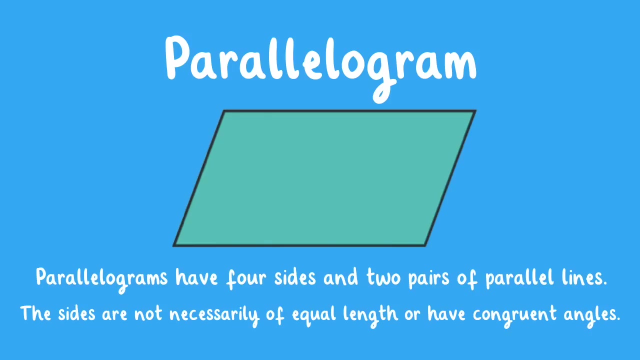 are the same in a regular octagon: Oval- Ovals only have one side and no corners. Rhombus A rhombus has four straight sides and four corners. All of the sides are the same length. Parallelogram: Parallelograms have four sides and two pairs of parallel lines. 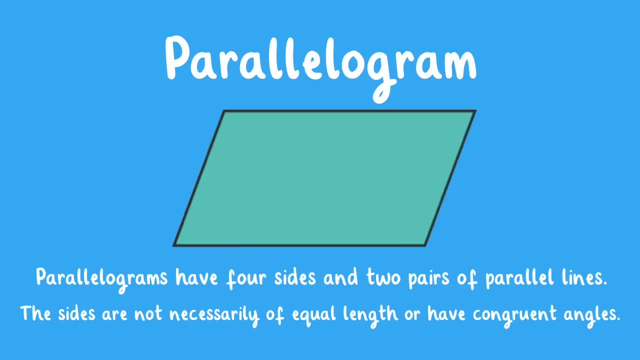 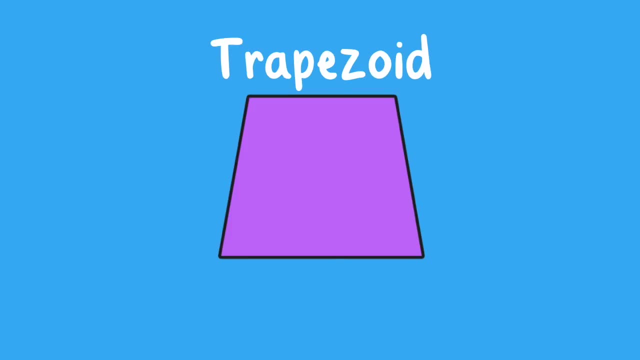 The sides are not necessarily of equal length or have congruent angles. Trapezoid: A trapezoid has four straight sides and four corners. It has two long sides and two short sides. Now that we've learned a few 2D shapes, let's move on to 3D shapes. 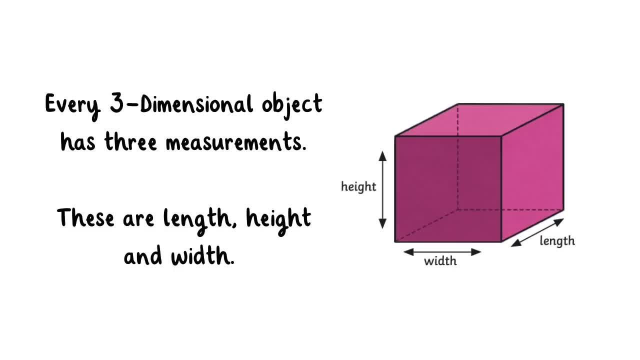 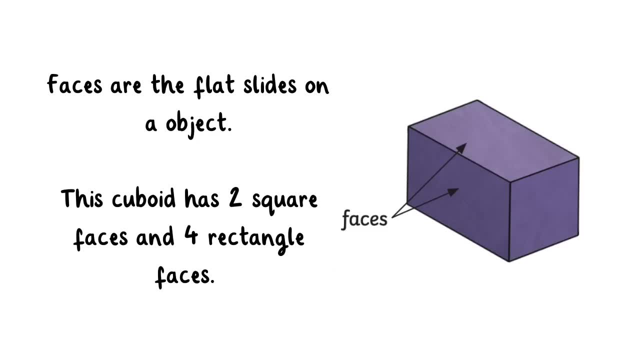 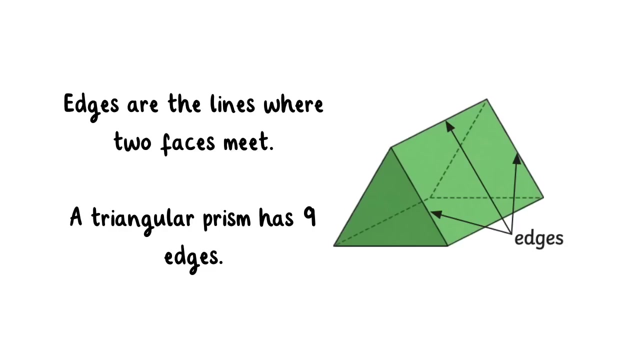 Every three-dimensional object has three measurements. These are length, height and width. Closest last ninth Faces: Facies are the flat sides on an object. This cuboid has two square faces and four rectangle faces. Edges are the lines where two faces meet. A triangular prism has nine edges. 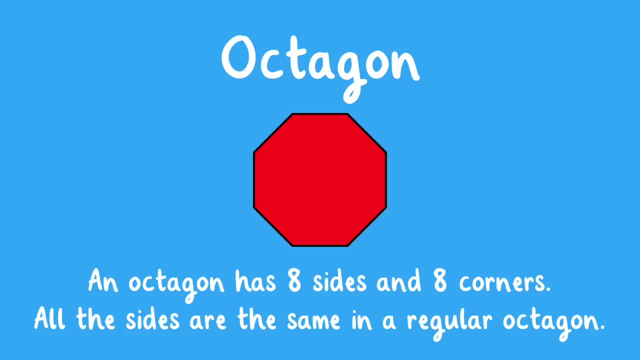 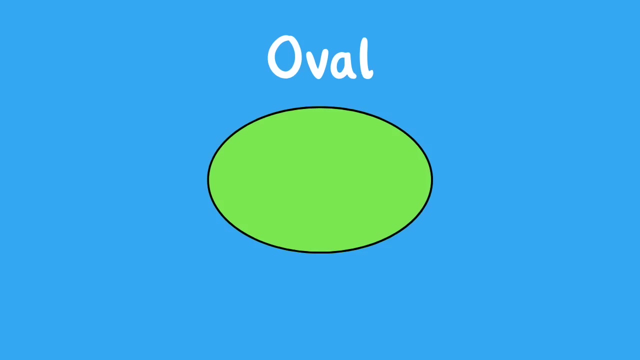 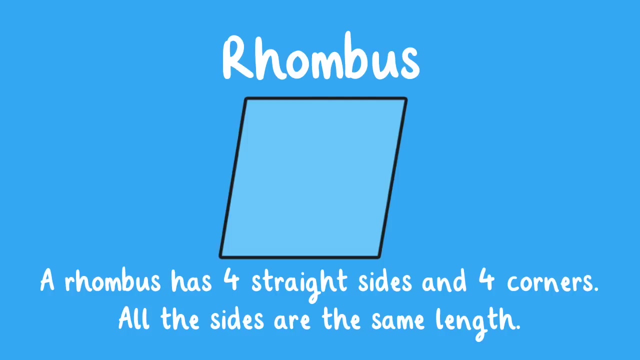 Octagon. An octagon has eight sides and eight corners. All the sides are the same. in a regular octagon, Oval, Ovals only have one side and no corners. Rhombus, A rhombus, has four straight sides and four corners. All the sides are the same length. 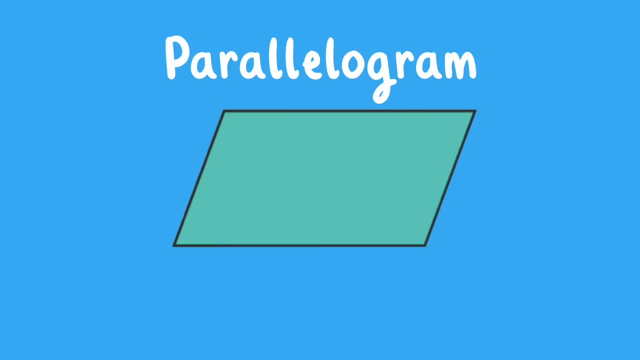 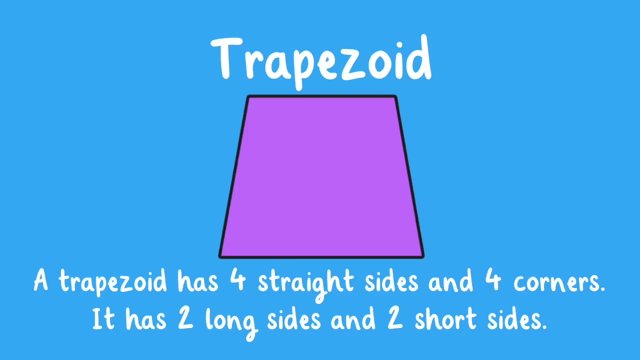 Parallelogram. Parallelograms have four sides and two pairs of parallel lines. The sides are not necessarily of equal length or have congruent angles. Trapezoid: A trapezoid has four straight sides and four corners. It has two long sides and two short sides. 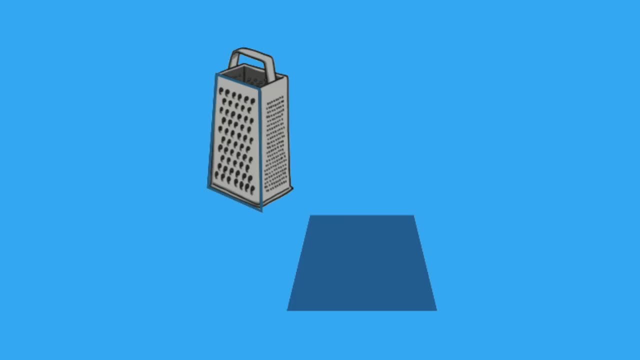 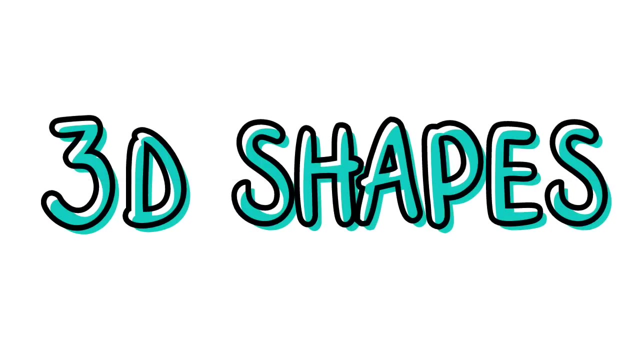 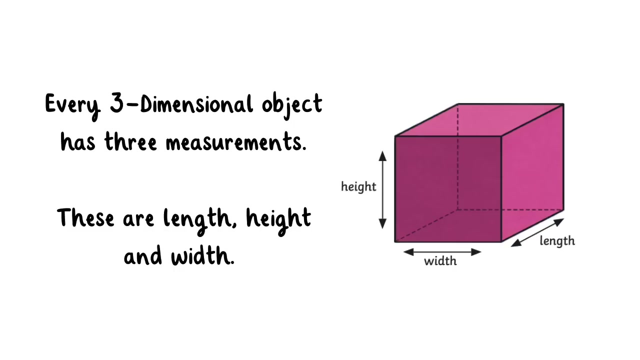 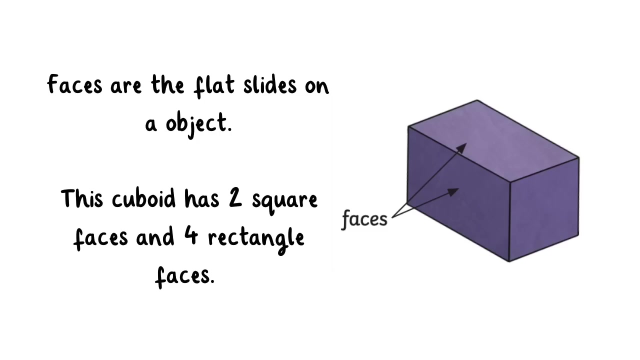 Triangular. Now that we've learned a few 2d shapes, let's move on to 3d shapes. Every three-dimensional object has three measurements. These are length, height and width. Faces are the flat sides on an object. This cuboid has two square faces. 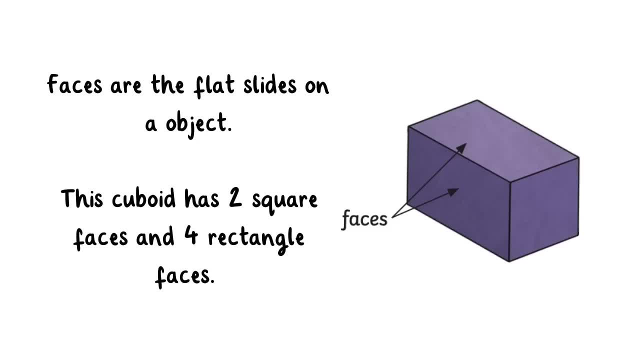 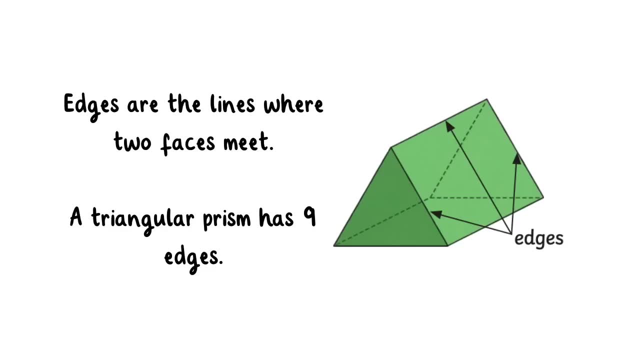 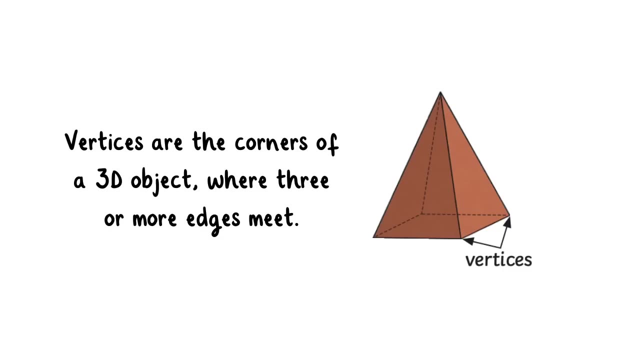 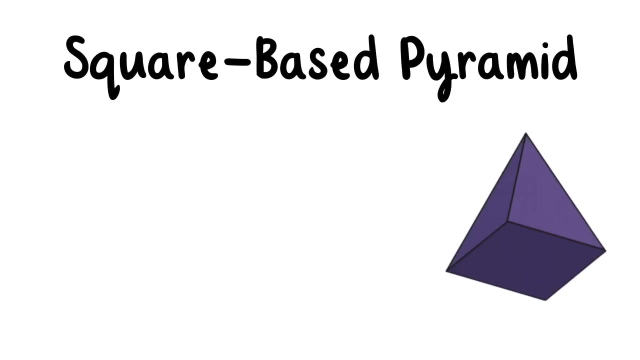 faces and four rectangle faces. Edges are the lines where two faces meet. A triangular prism has nine edges. Vertices are the corners of a 3D object where three or more edges meet. This is a square-based pyramid. Square-based pyramids have a square base, four triangular. 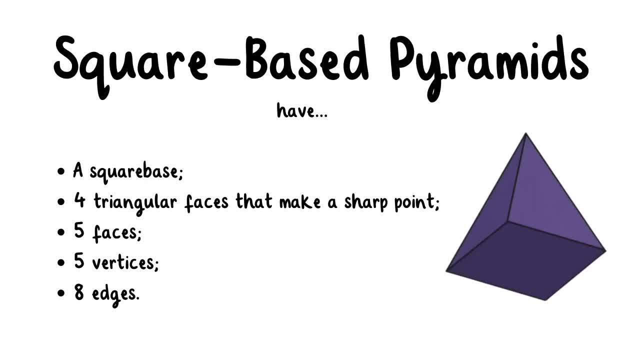 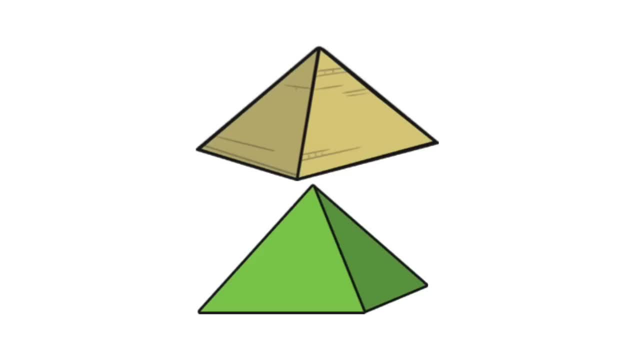 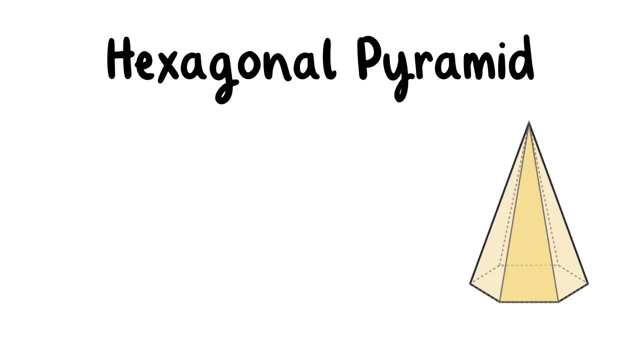 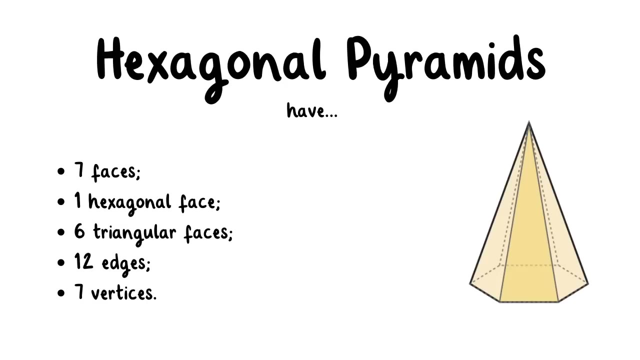 faces that make a sharp point: five faces, five vertices and eight edges. Here's a real life example. This is a hexagonal pyramid, Hexagonal pyramid. Hexagonal pyramids have seven faces: one hexagonal face, six triangular faces, twelve edges. 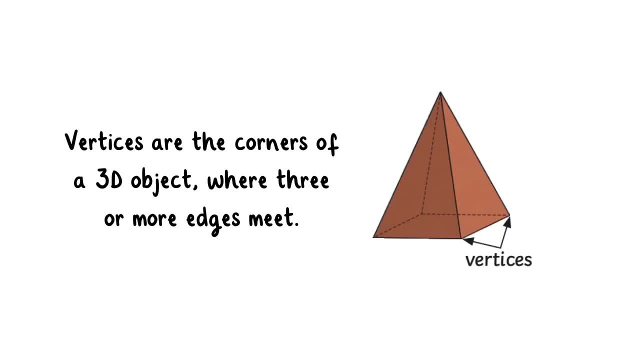 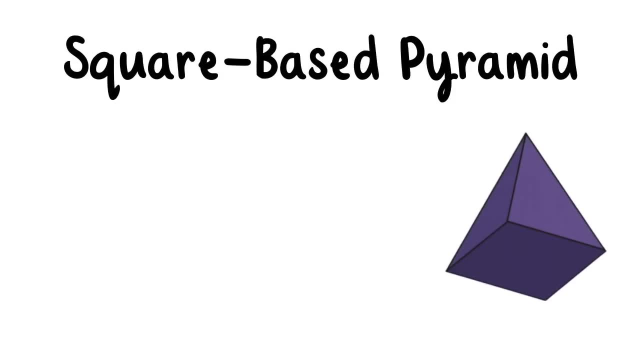 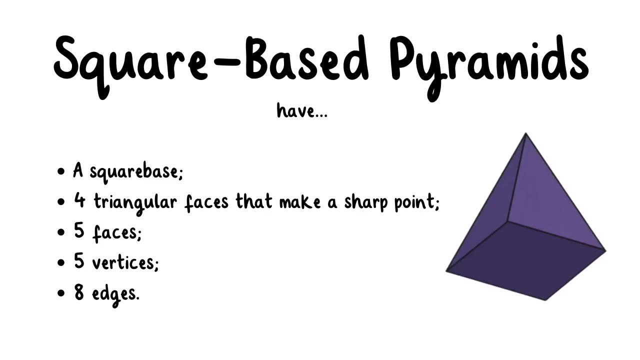 Vertices are the corners of a 3D object where three or more edges meet. plane is a square-based pyramid. Square-based pyramids have a square base, four triangular faces that make a sharp point, five faces, five vertices and eight edges. 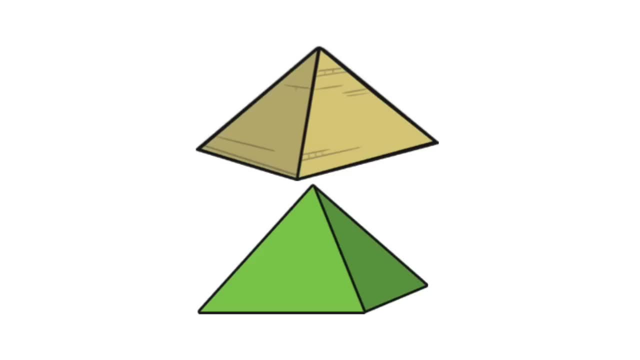 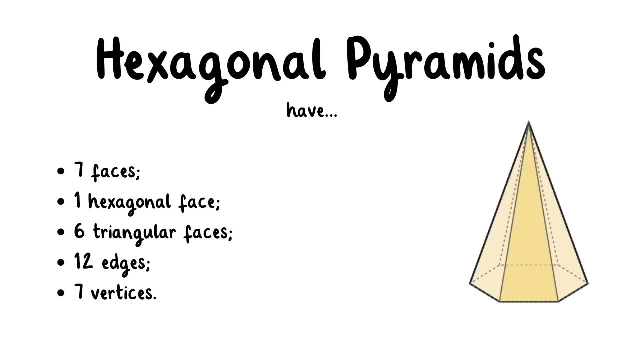 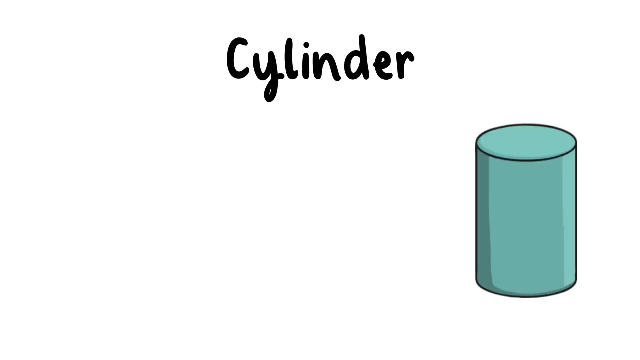 Here's a real life example. This is a hexagonal pyramid. Hexagonal pyramids have seven faces: one hexagonal face, six triangular faces, twelve edges and seven vertices. This is a cylinder. Cylinders have two flat and circular faces, one curved surface no vertices and two curved edges. 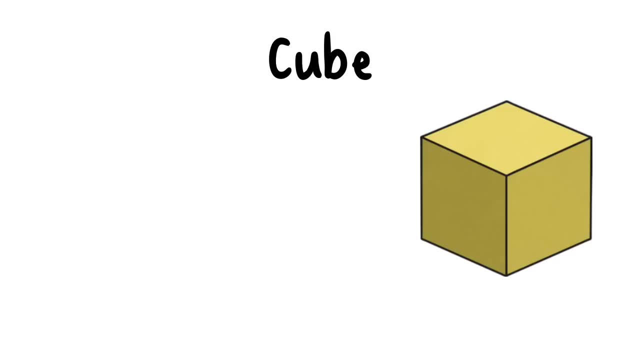 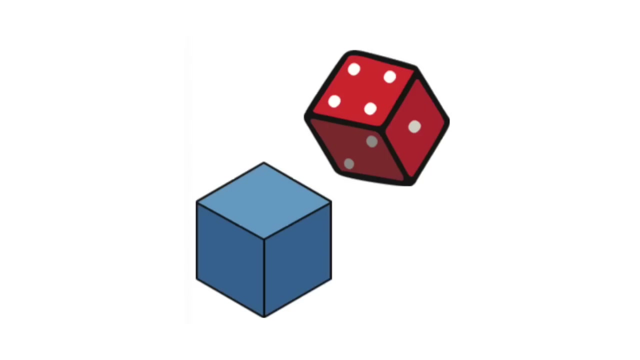 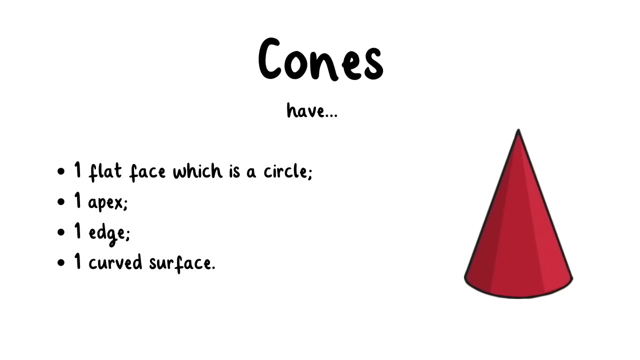 This is a cube. Cubes have six square faces, 12 edges, eight vertices and edges that are all the same length. This is a cone. Cones have one flat face, which is a circle, one apex, one edge and one curved surface. 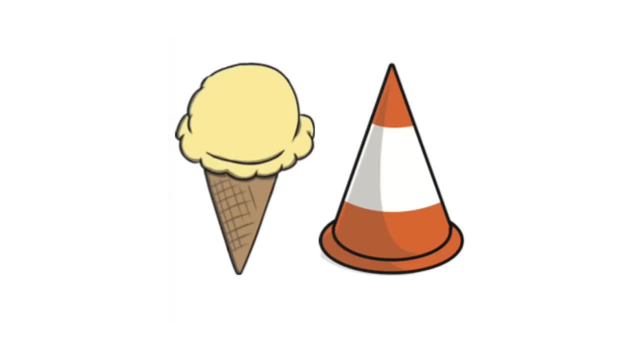 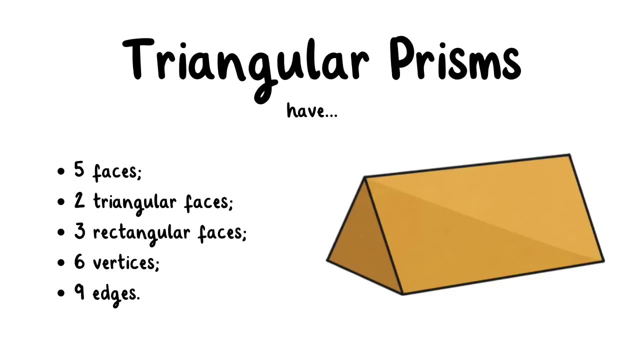 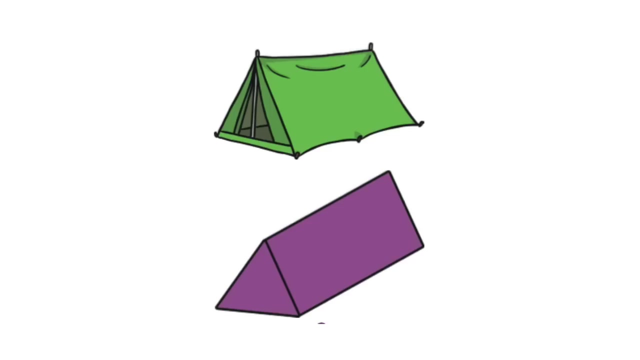 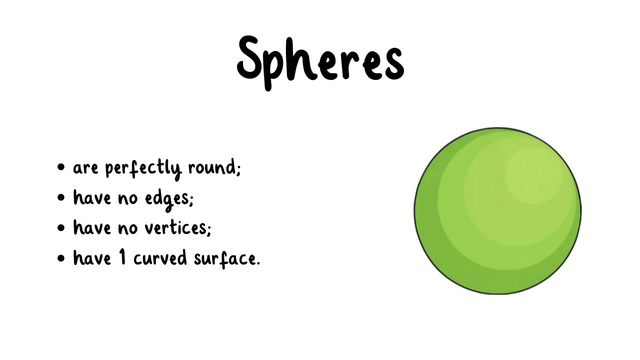 This is a triangular prism. Triangular prisms have five edges, one curved edge and one curved surface. Five faces: two triangular faces, three rectangular faces, six vertices and nine edges. This is a sphere. Spheres are perfectly round, have no edges, have no vertices and have one curved surface. 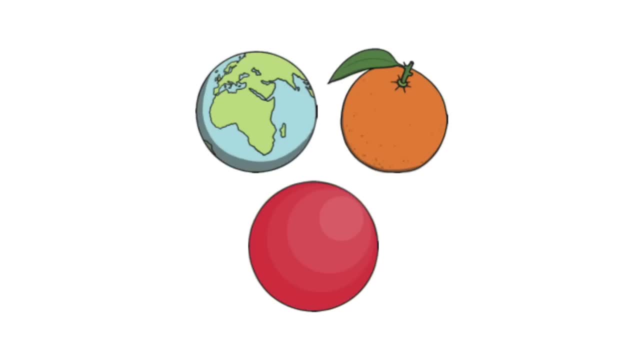 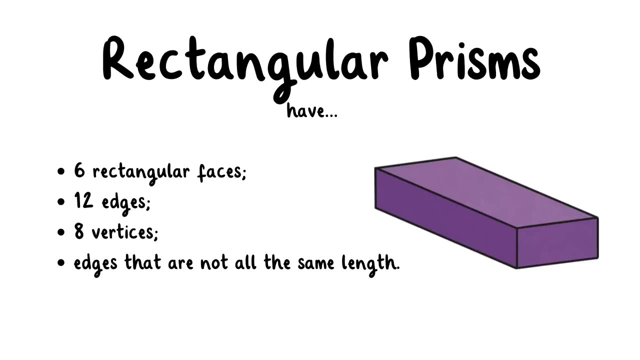 This is a star flower. The color is 충light green, The interior is gray, a little drop of color and white. This is a watermelon Terminal, number 10.. A little identifier of the relates this to aмara tree is an otherwise específic statement.